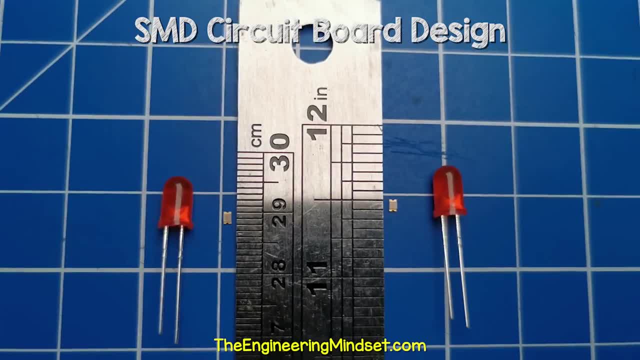 Here you can see it's a 3.5 volt battery. I'll zoom in so you can see it. Here you can see it's a 3.5 volt battery. I'll zoom in so you can see it Next to a scale, so you can really see just how tiny these components are. 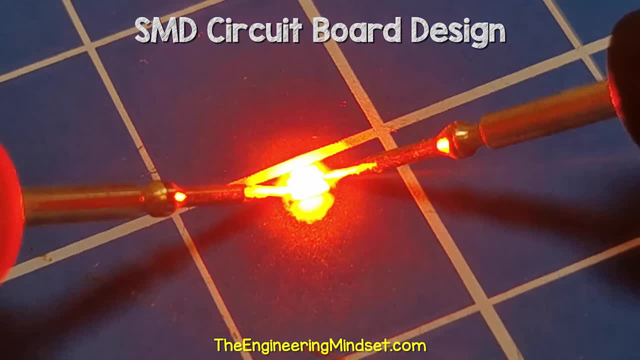 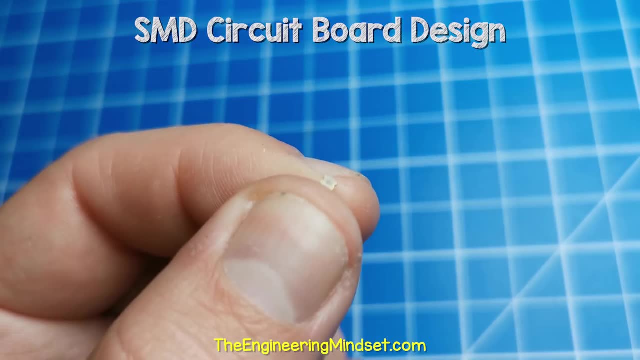 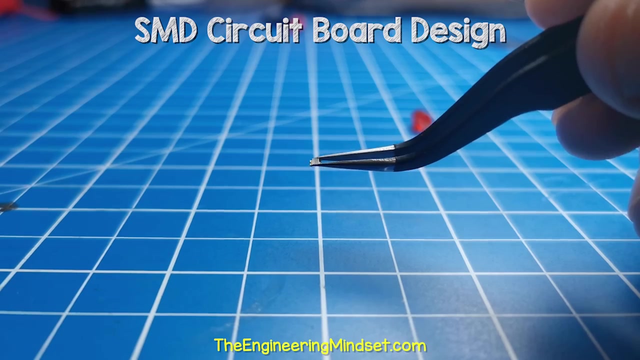 However, it can produce a good amount of light, So I will use five of these, as that will keep the circuit board simple, but also fairly small. The SMD LEDs are tricky to handle, so you'll need some tweezers for that. My top tip is to handle them on a flat, dark colored surface. 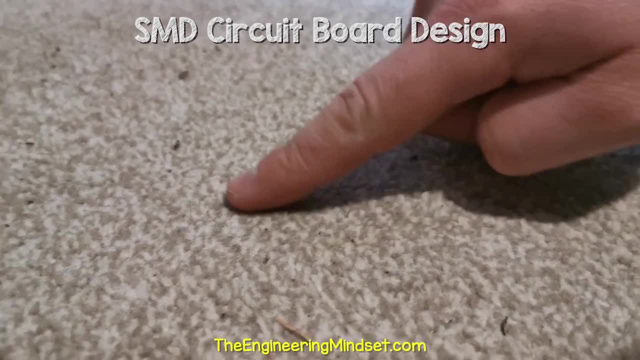 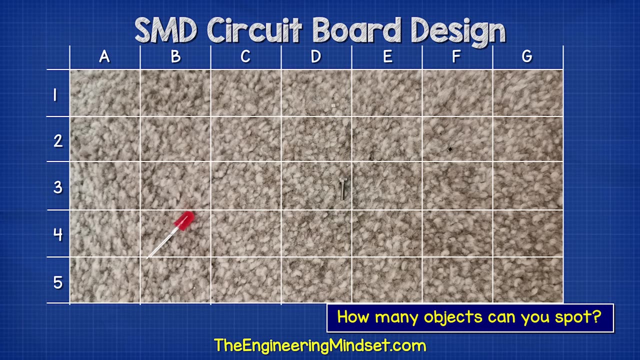 because if you drop them on a carpet, you're probably never going to find them again. As a quick test, how many objects can you see in this carpet? Tell me the grid reference for them and let me know your answers in the comments section down below. 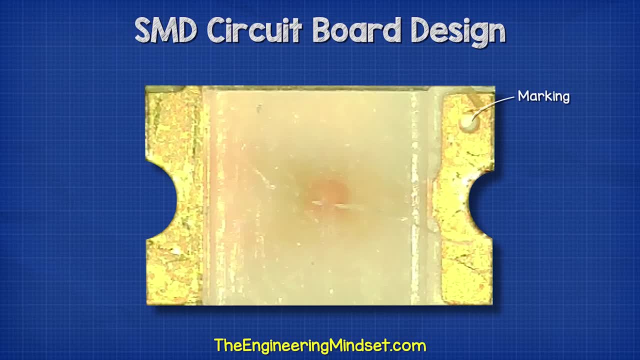 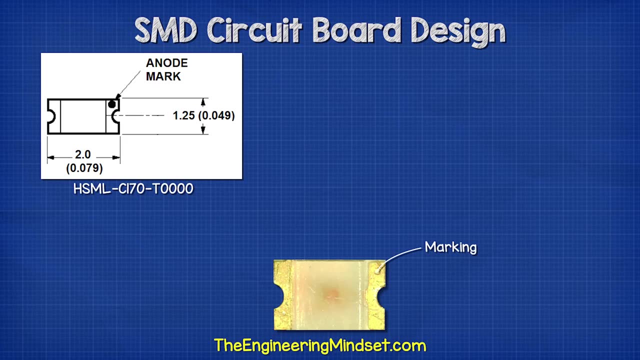 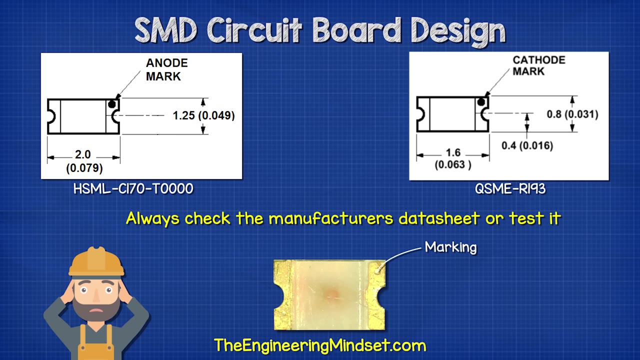 The SMD LED typically has a small dot on the top, although you might need a microscope to see this, But sometimes the manufacturer uses this to indicate the anode and other times it's used to indicate the cathode. So always check with the manufacturer's data sheet or you can test it. 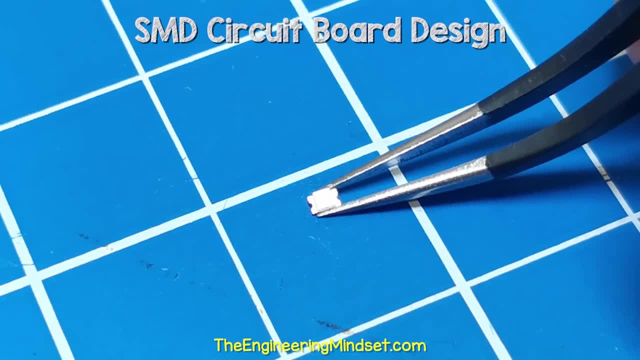 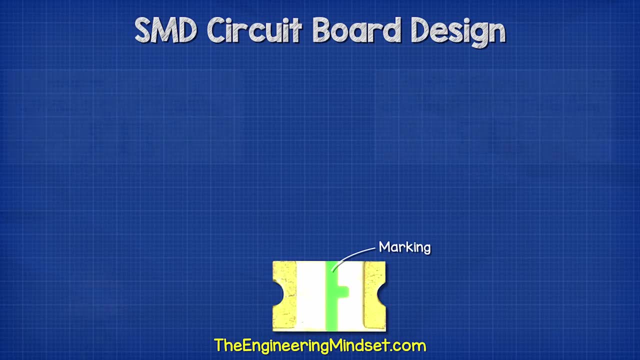 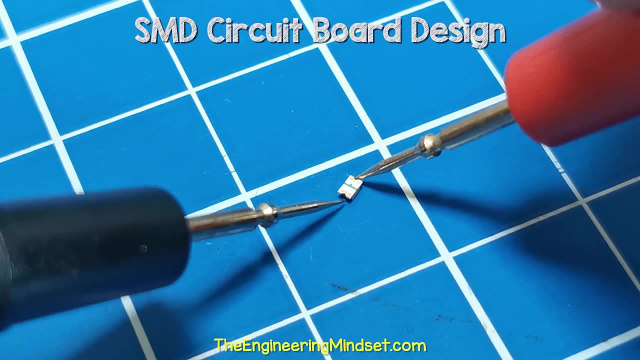 yourself. Here you can see that this LED illuminates when the positive is connected to the dot On the back. you should find a symbol also. Again, this could be either the anode or the cathode. So check the data sheet or test it. Here we can see the LED illuminates when it's connected like: 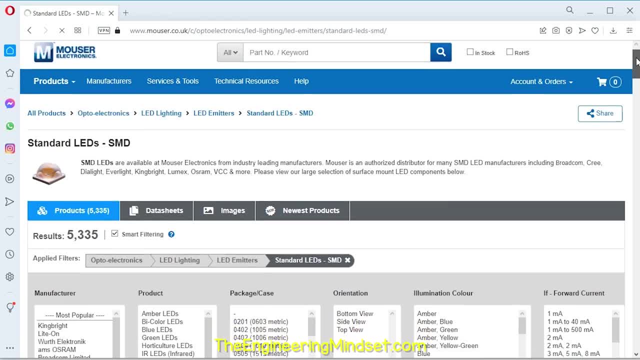 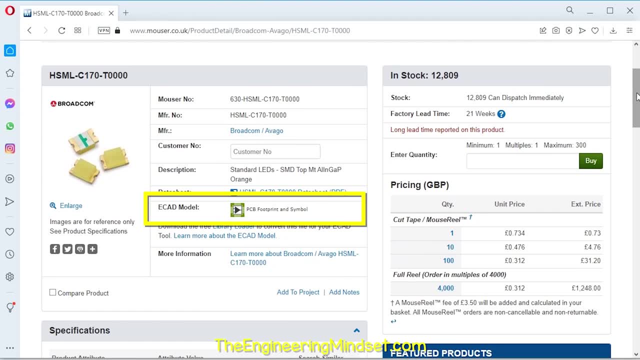 this. To find the LED, we're going to go to a supplier's website and search through their components. I like these ones because they have a PCB footprint which is a little bit more accurate. They're not quite as smaller, but they expand and look a lot better. 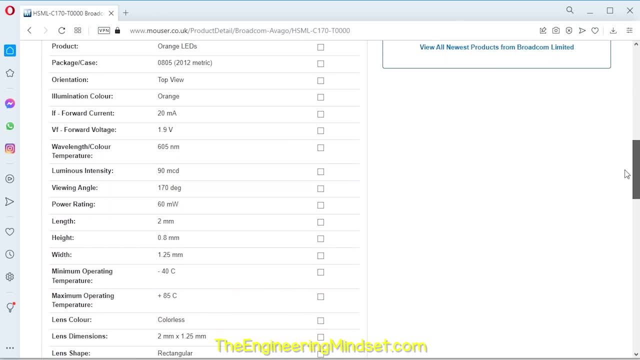 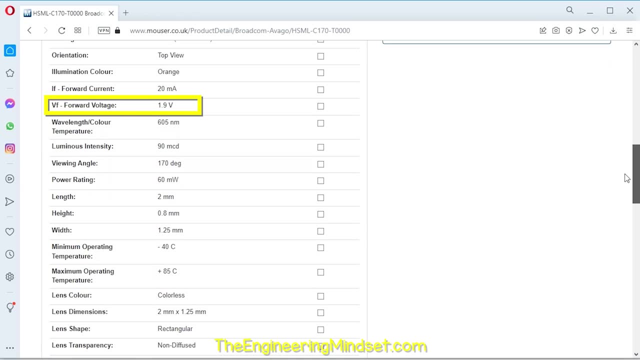 Alternatively, try going over my demo. Even if these only have the same number ofľs connected to a signal, we can exactly tell they're from a different circuit. Teacher, I not be guilty in needing a new one to test the DC Colon As the LED tries to be connected? we can now look for a current. 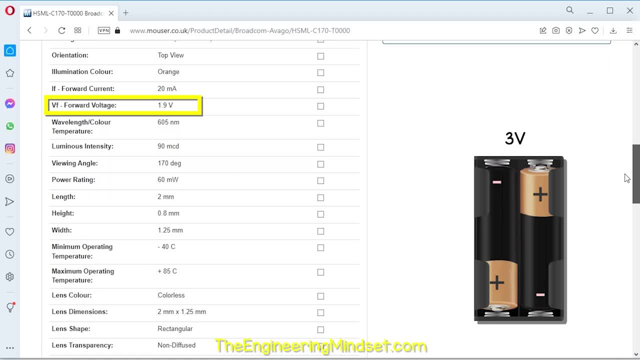 Which we can see. that shall be round and a bit bigger. This LED supports the LED in aillar, As you see that thousand volts have been added. If we can connect it, in what level ofй? It would be the one that will allow the cycle to Romania that is set togther. 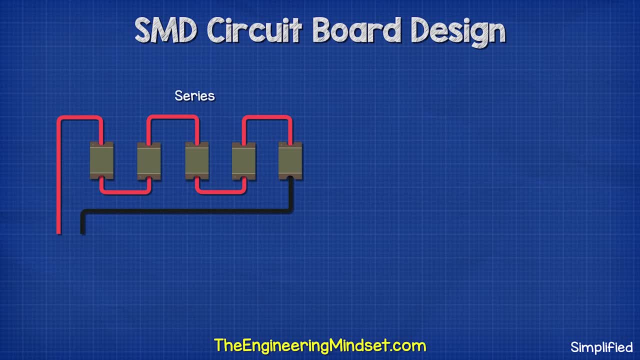 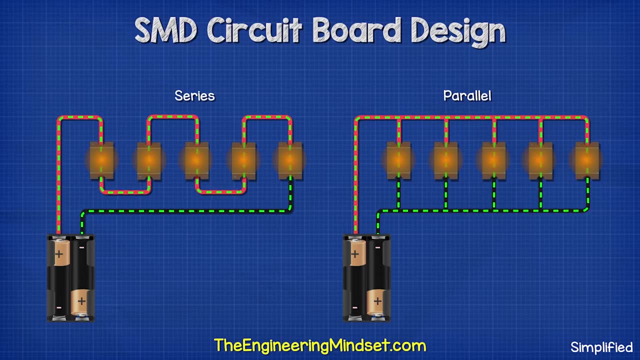 In this case SE4 times of67,se rzecz. xtIt has grown to 20mA. It will give us the frickest use we have to pay for the grid compared to the other LED's. If we connect them in series, then each LED is going to remove an additional 1.9 volts, so that 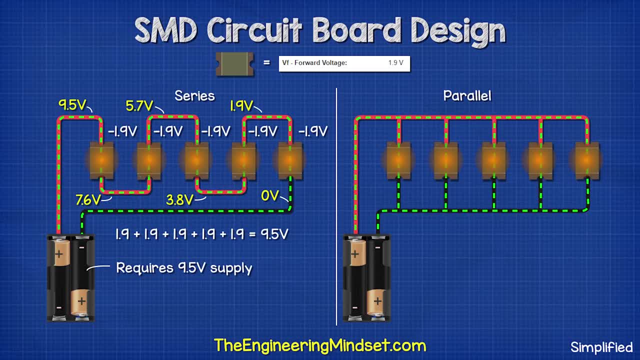 means we need around 9.5 volts of power supply to the circuit board to be able to power them all, so we can't use this method. We will instead connect them in parallel so that each LED receives the same voltage. Then we would only need a supply of 1.9 volts. however, we will be 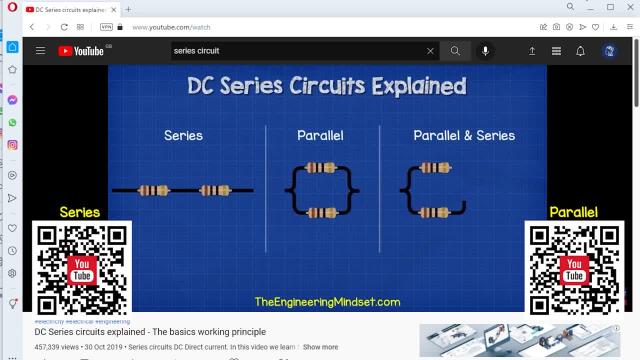 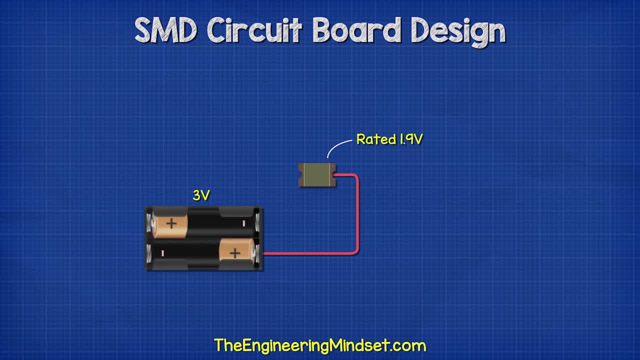 using the 3 volt supply. By the way, we have covered series and parallel circuits in detail in our previous video. Links down below for that. Now, if we provide an LED with 3 volts and it's only rated to handle 1.9 volts, then we're going to destroy it. Too much current is going to flow. 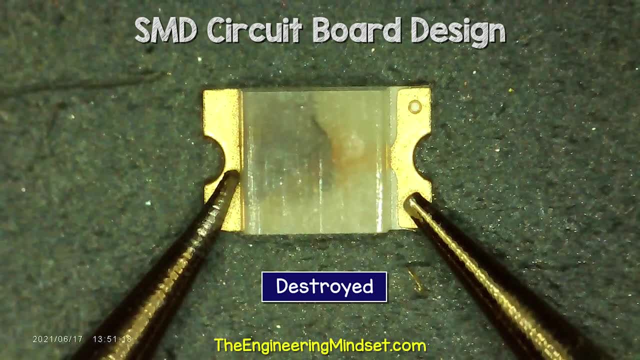 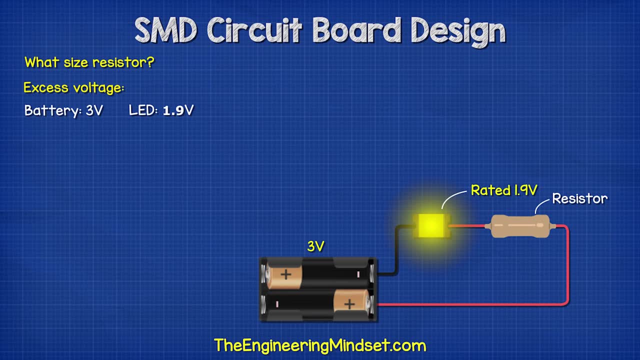 through the component and it will burn out. so we need a resistor to limit the current and remove that excess voltage. What size resistor do we need? Well, we have a 3 volt supply and the LED has a voltage drop of 1.9 volts. so if we subtract this from the 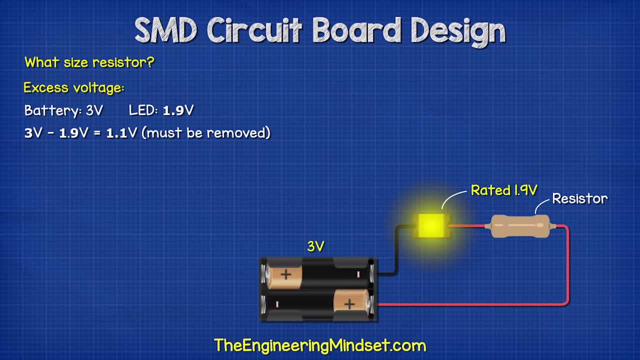 power supply. then we have to reduce the voltage by 1.1 volts. The LEDs are rated for 20 milliamps or 0.02 amps. so 1.1 volts divided by 0.02 amps gives us a resistance of 55 ohms. and, by the way, 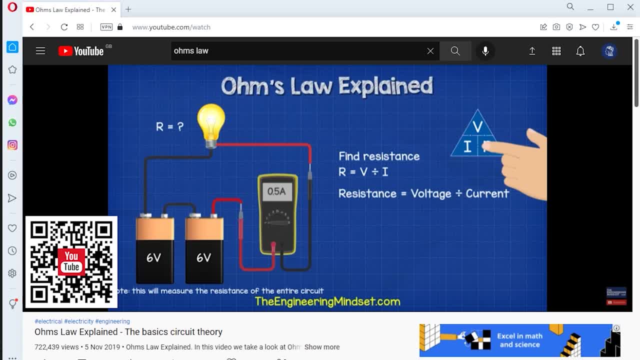 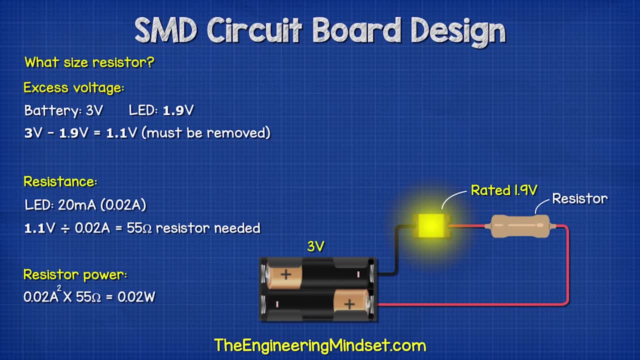 we have also covered Ohm's law in DC, So we will need to know the power rating of the resistor. We calculate that from the current of 0.02 amps squared, multiplied by 55 ohms, which gives us 0.022 watts, and that is a very small. 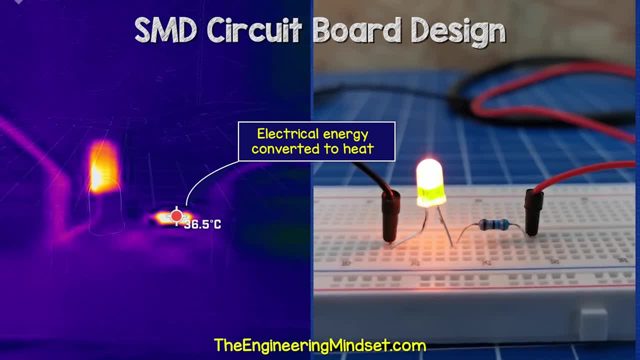 amount, which is a good thing, because that's how much energy we're wasting as heat from the resistor. To remove that excess 1.1 volts, we basically convert the energy into the resistance into heat to remove it. Okay, so we want to use SMD components. 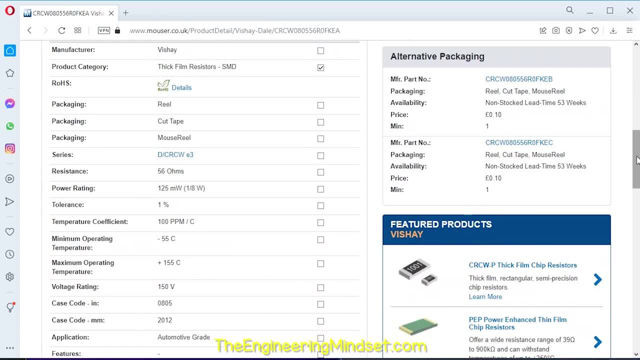 so we search the supplier website and I will use this one. It is rated for 56 ohms, so it's slightly higher than we need, but close enough. It has a tolerance of 1%, meaning it could be anything between 55.44 ohms. 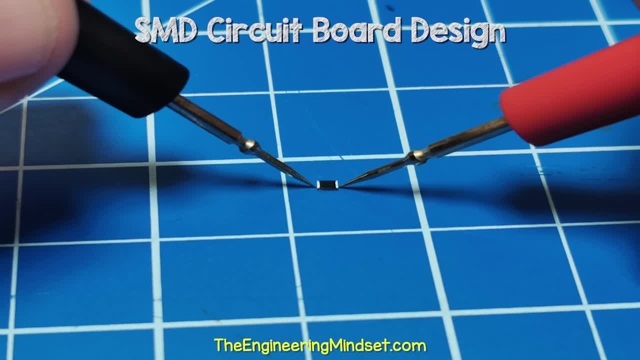 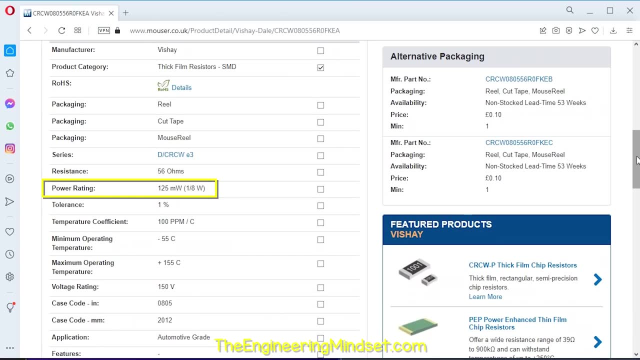 or 56.56 ohms. When I test this one, it's showing 56.3 ohms. We can also see that this resistor is able to handle up to 125 milliwatts, which is much higher than our 22 milliwatt design. 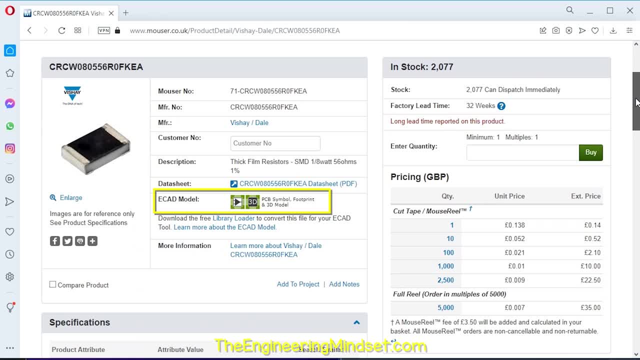 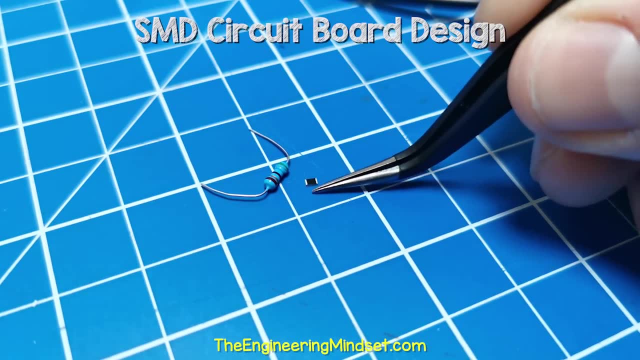 And this component also has a drawing as well, which we can use in our design, So we will use this component. These resistors are also incredibly small, so you'll need some tweezers to handle them. We don't need to worry about the polarity. 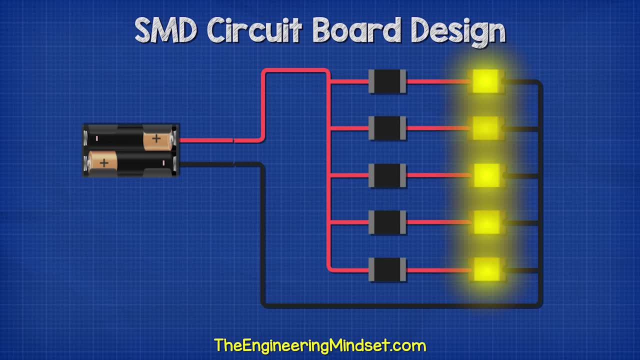 because they will work either way. we connect them. So we have five LEDs in parallel with a resistor connected to each one. Next, we need a way to connect the battery pack to the circuit. We could just solder them, but I'm going to use a terminal block. 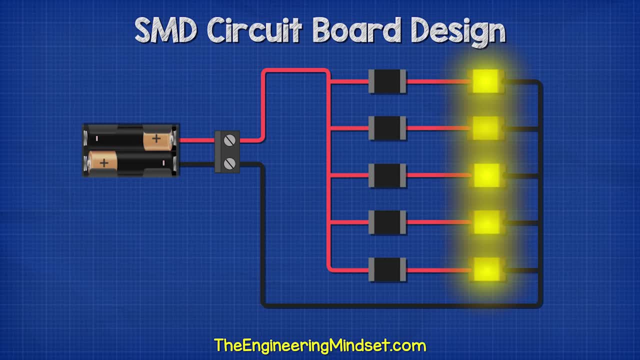 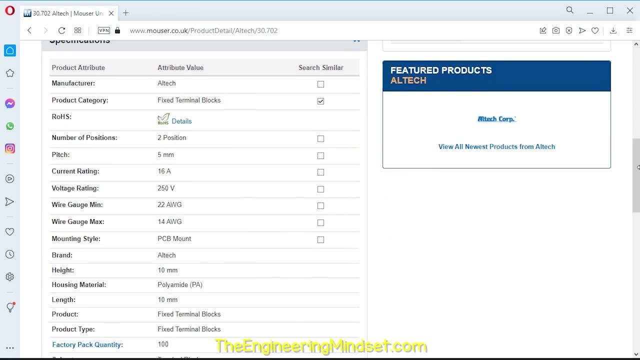 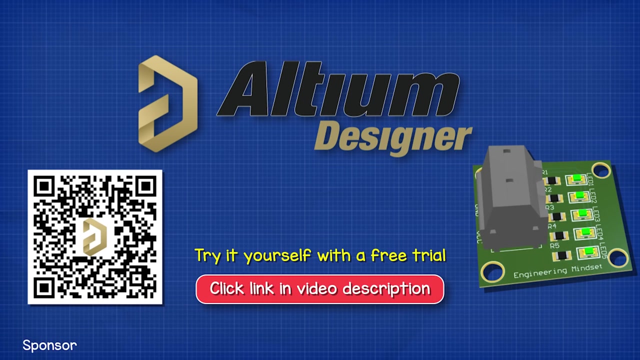 so that we can easily connect to different power sources in the future if we needed to. We only need a positive and ground connection, so we will use this model right here Now. to design the circuit board, We're going to be using Altium Designer. 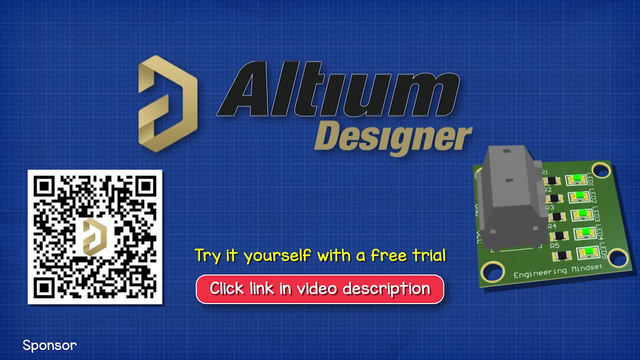 who have kindly sponsored us to do this video. All of our viewers can get a free trial of the software, and I will leave a link for you in the video description down below. so do check that out. So we start a new project. 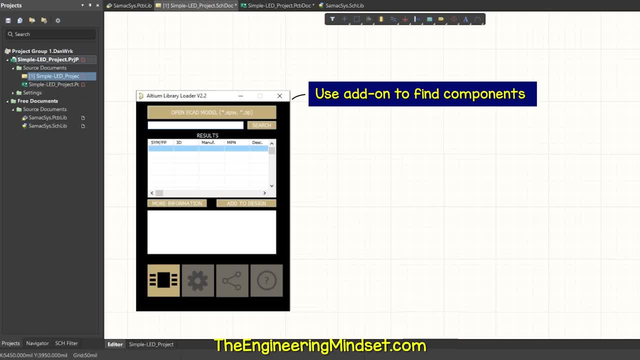 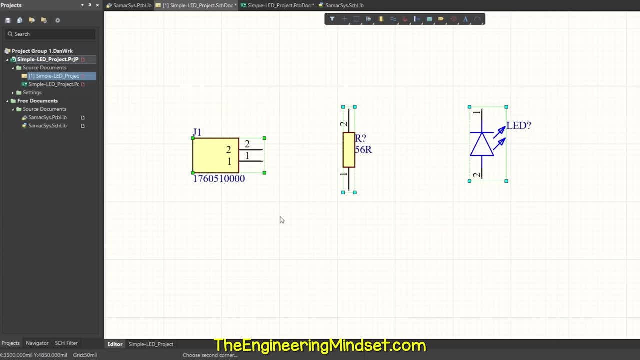 and then we add in the symbols of the components we found. I use an add-on to do that, just input the part number. We only have three components: the LED, the resistor and the connector. We join the LED and resistor. 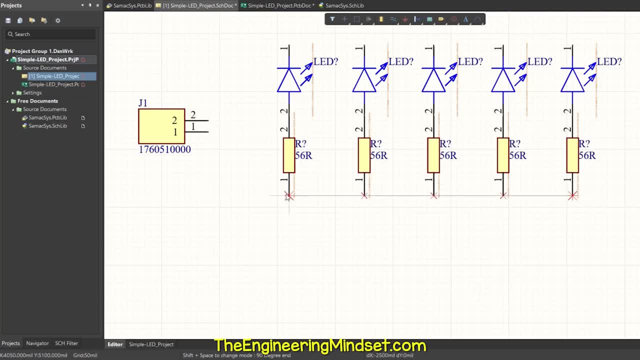 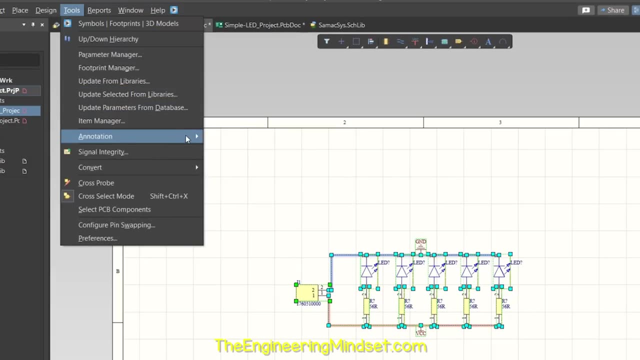 and then we duplicate it. Then we connect the resistors and then we join it to the connector. Then we connect the LEDs together and we join that to the connector also. Then we define the ground and positive points of the circuit. Next we just add some annotations to the board. 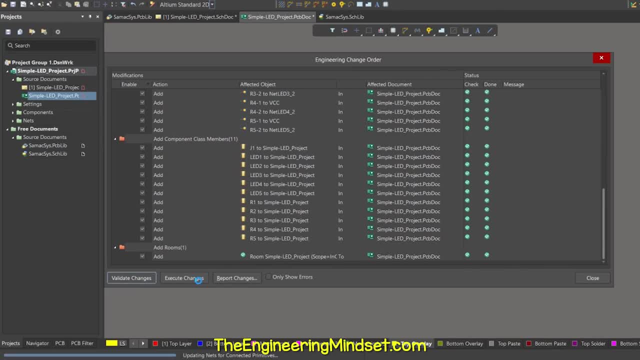 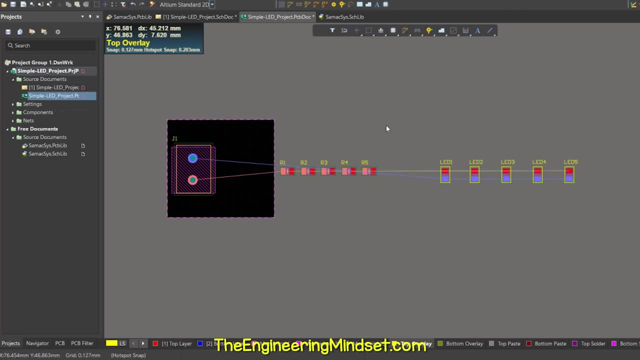 and then go to the PCB layout and import the components, Drag the connector into place. I'd also say check it in 3D to ensure it's facing the correct way and then move the LEDs to the right and then move the LEDs into position and align them. 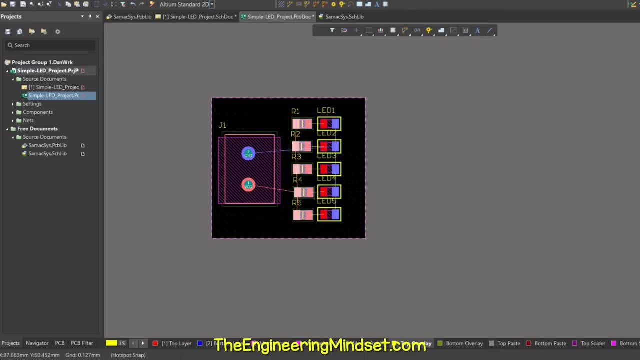 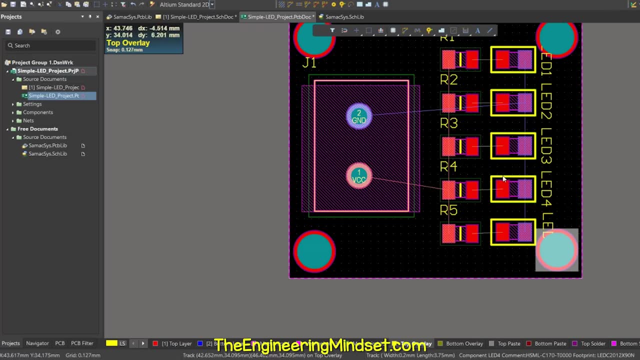 Next, move the resistors into place and align them. also, You can move the text if you wish. I'll also add some holes so that we can mount the circuit board in future if we needed to, and then I'll adjust the position of the components. 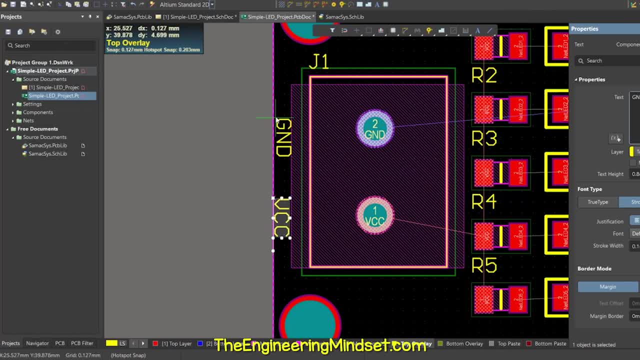 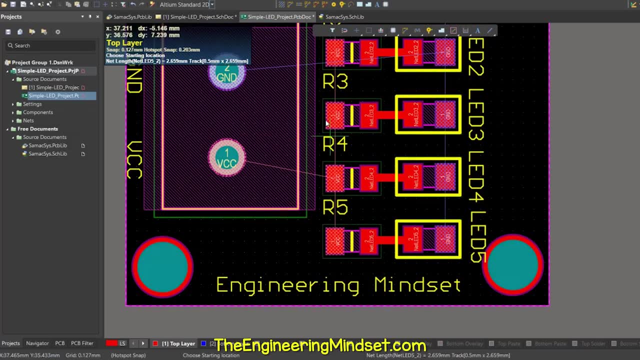 Then we just define the positive and ground ports on the board, And now we start to draw the routes between the components. We connect the resistors and the LED first, then all the resistors too, and then the connector together and connect that to the positive port. 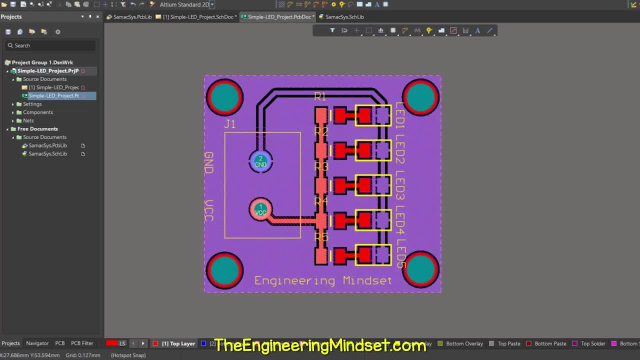 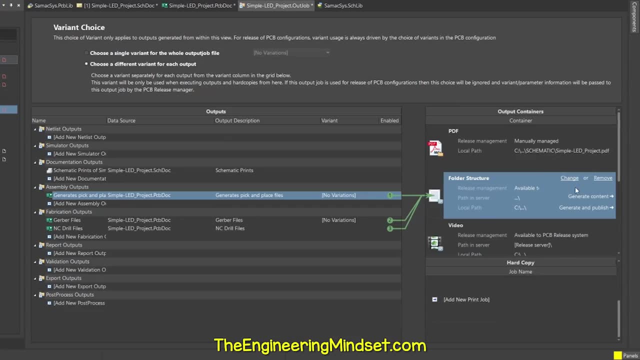 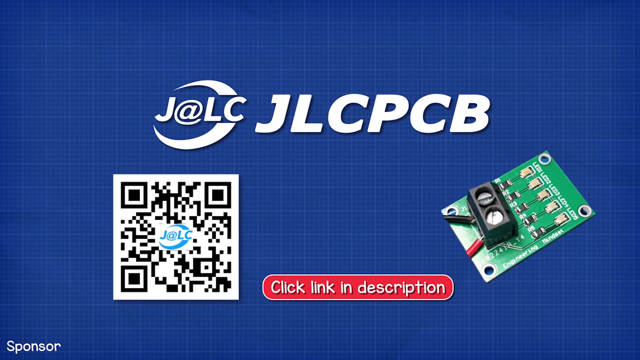 Then connect all the LEDs together and connect them to the ground port. Finally, set your polygon and the PCB now looks like this, So we can export the project. To order the PCB, we just head to JLC PCB, who have also kindly sponsored this video. 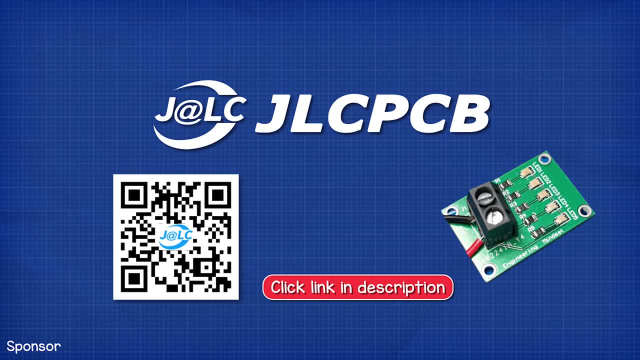 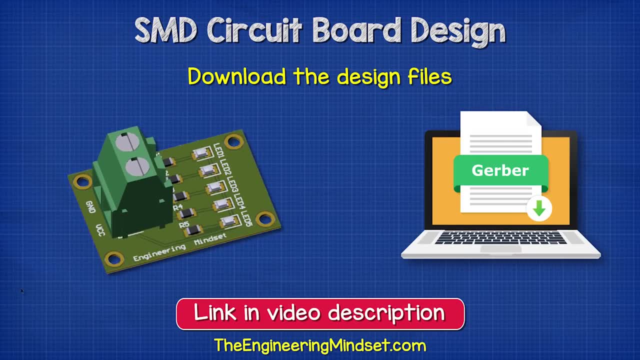 They offer exceptional value with five circuit boards from just two dollars. I'll leave a link for you in the video description down below. Do check that out. And also don't forget, you can download my circuit board design file for free. links down below for that. 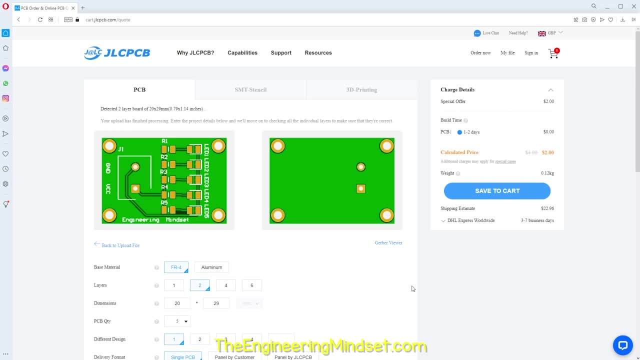 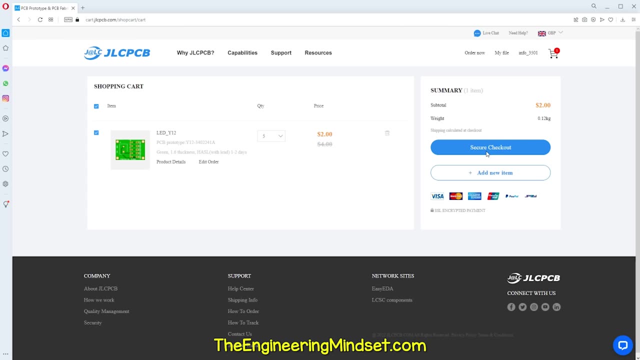 So we upload our Gerber files and check the preview. It looks good. So we can then set the color, although I will stick with green, and then I'll head to the checkout. a few days later Our circuits arrive in the post and we can start building the circuit. 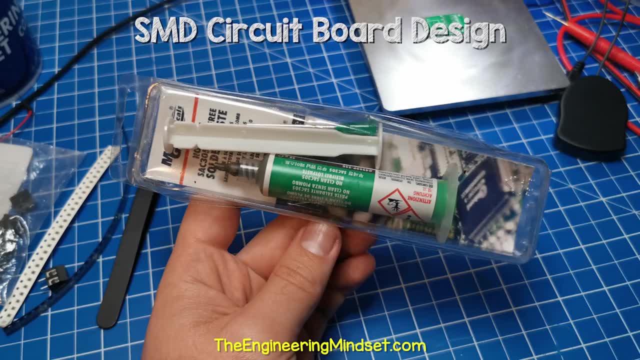 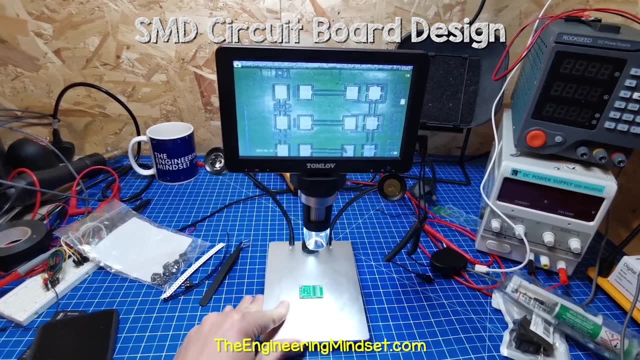 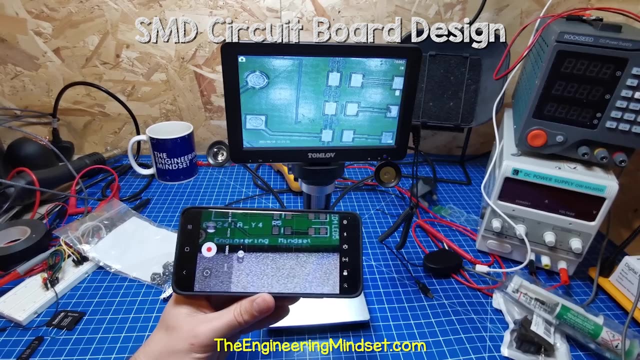 So get your components ready. We will use some solder paste and you can buy this online. I will leave a link for you in the video description. Now, unless you have incredible vision, which I do not, you will need a microscope or you could use your smartphone to zoom in and see the board and components. 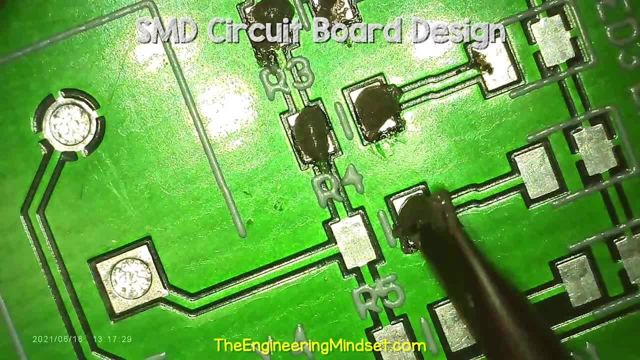 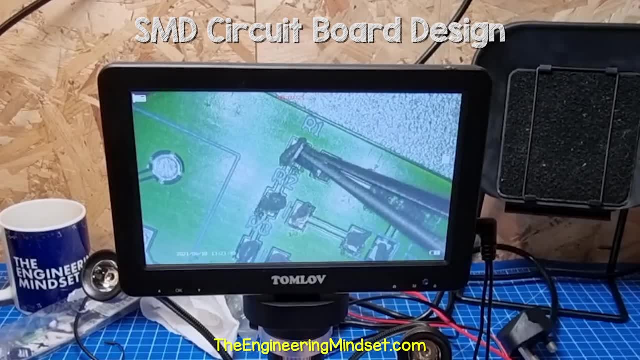 So all we need to do is put a small amount of paste onto each of the solder pads on the board. Then we start to add the components. I'll add the resistors first, as they are the easiest. You'll need some tweezers to get them. 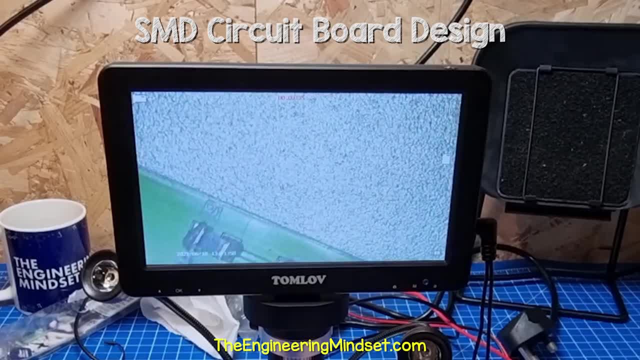 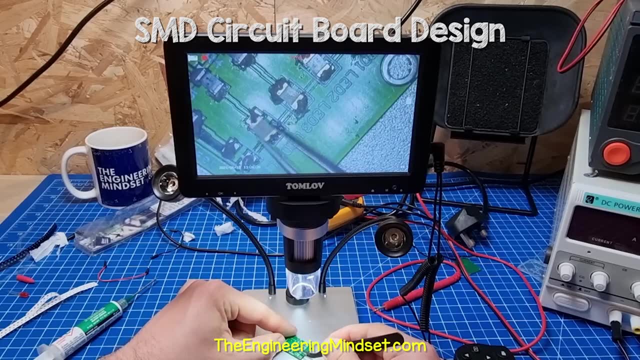 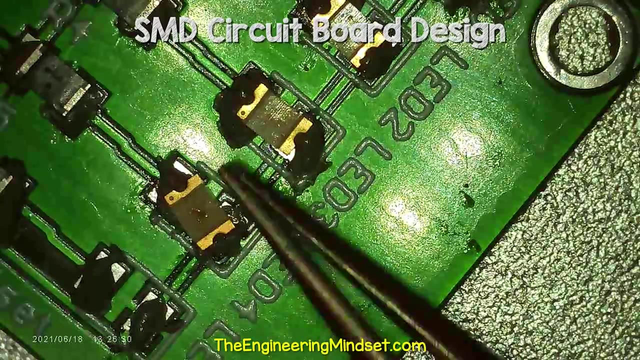 positioned correctly and also push them into the paste, And then it should look something like this. Now for the LEDs. make sure you align them correctly, And to do that you'll need to check the manufacturer's data sheet. So we just align the LEDs the correct way until it looks something like this: